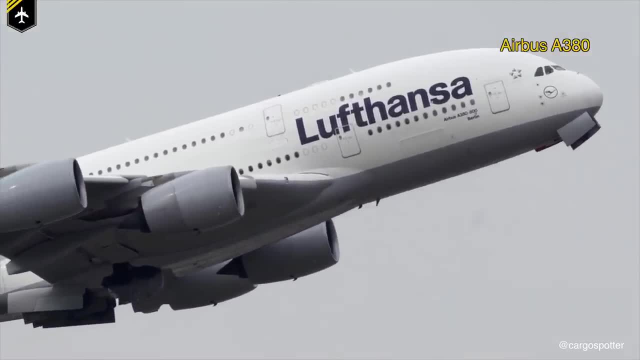 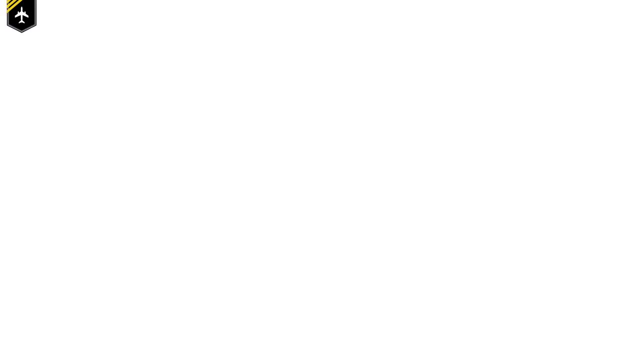 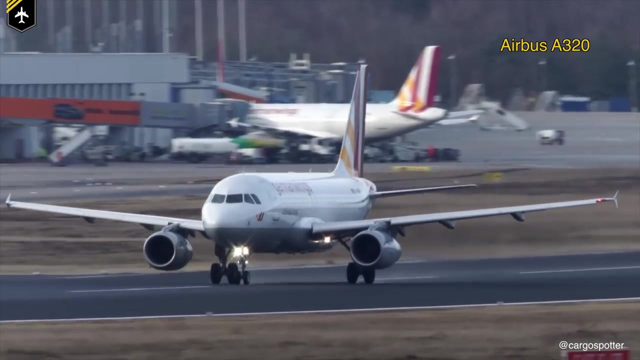 much rounder Now, aerodynamically speaking, one isn't better than the other, It's just a coincidence that allows anyone who's interested to tell them apart, Depending on what view you have of the aircraft. another easy way to quickly spot the difference, specifically, between an Airbus from: 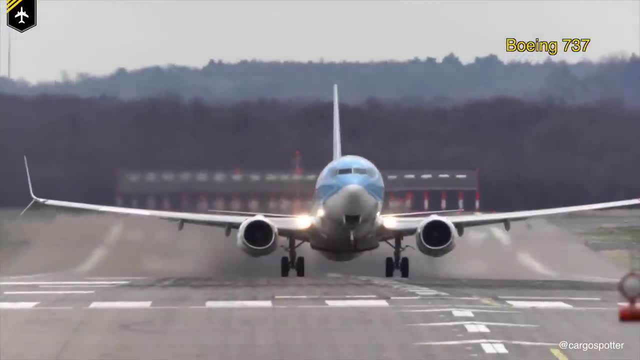 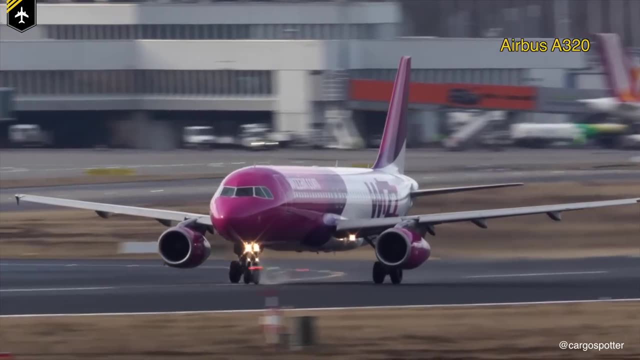 the A320 family and the Boeing 737, is to take a closer look at the nose of an Airbus. If you want to see the difference, you can take a look at the shape of the engine. Now, not many immediately notice the difference, but a closer inspection, the shape of the engine cowlings are quite 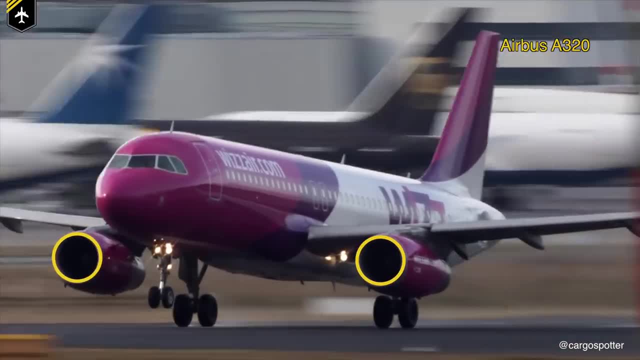 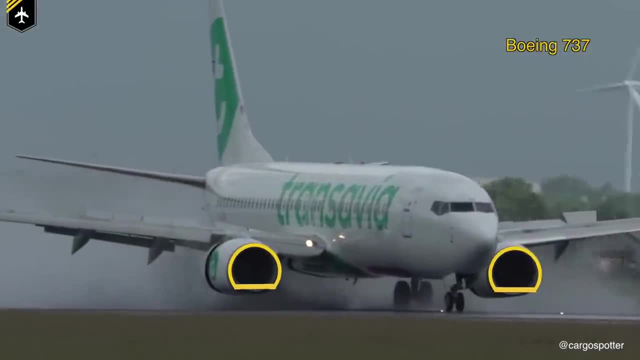 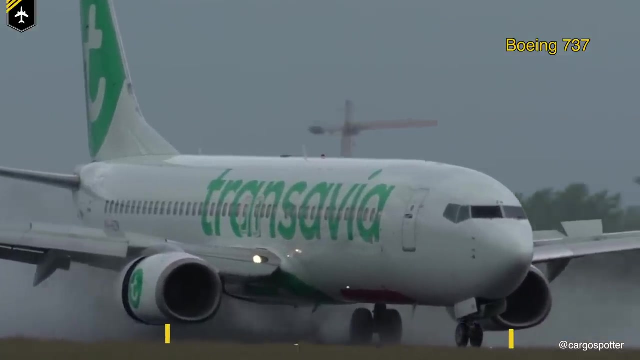 different. Airbus almost has a perfect circular shape. However, with a Boeing, you can spot that the bottom of the engine is not so perfectly circular and almost flat. You will also see that the actual engine of the Boeing 737 has very little ground clearance compared with an Airbus. 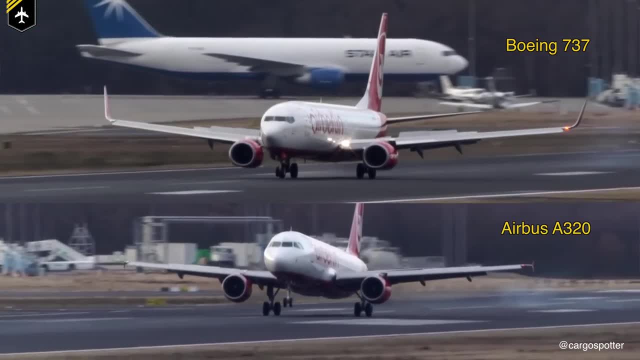 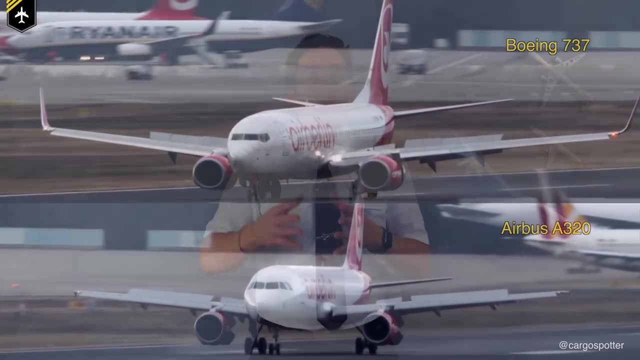 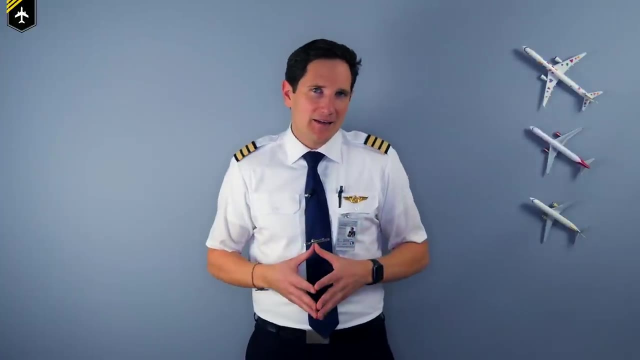 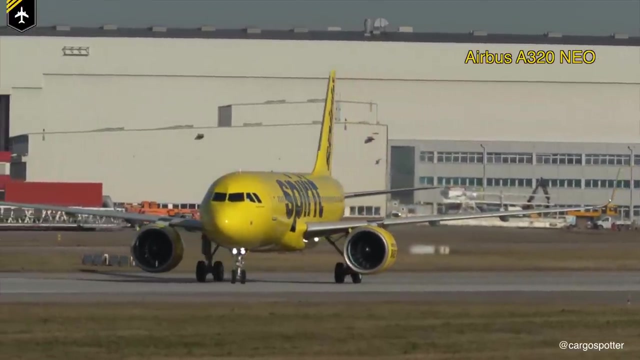 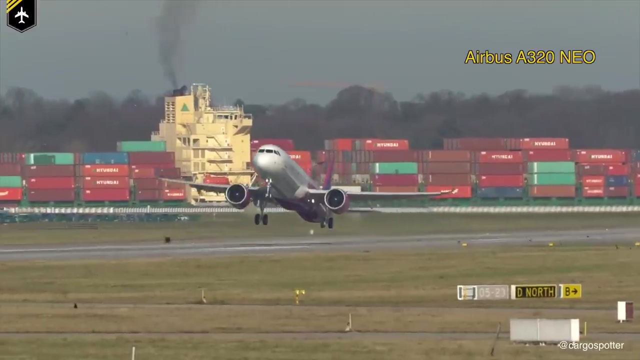 The design of the Boeing. in fact, has caused Boeing to completely redesign the landing gear for the new Boeing 737 MAX. Airbus haven't had this issue with the rollout of their new A320 NEO fleet and has allowed them to use much larger engines, which are far much more efficient, without having to worry about. 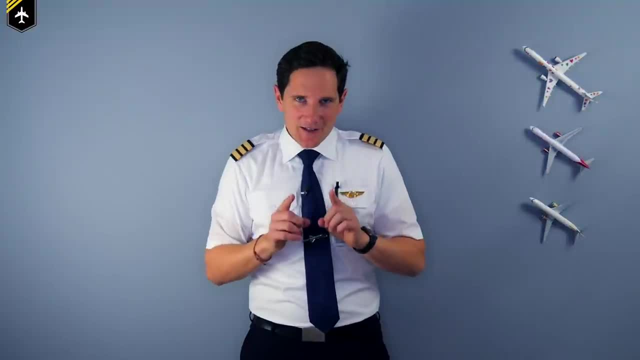 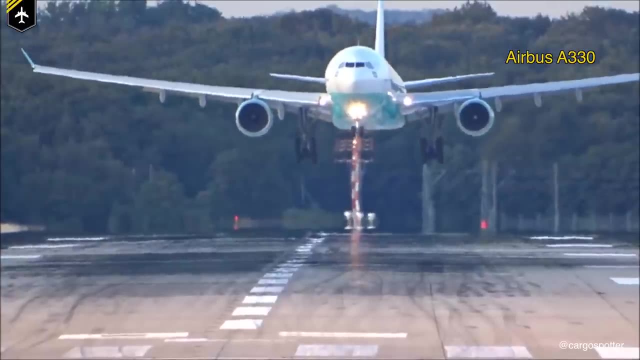 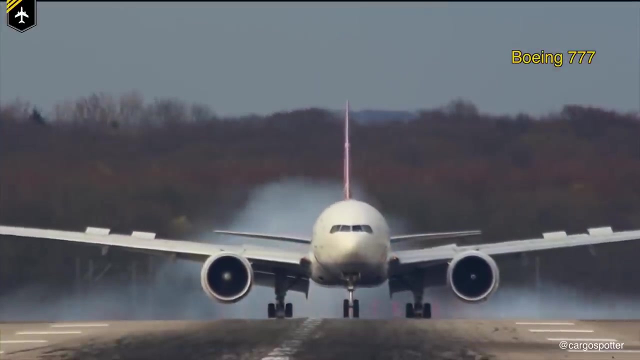 minimal ground clearance. Now to start spotting the differences between more specific aircraft. we are going to go into more details about some very iconic ones. How to tell the difference between an Airbus A330 and a Boeing 777?? Now, they are similar in size and shape. 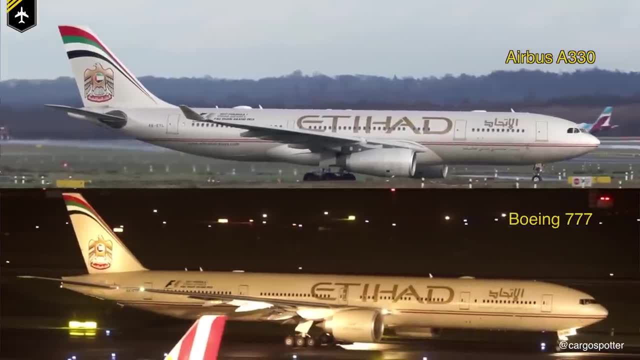 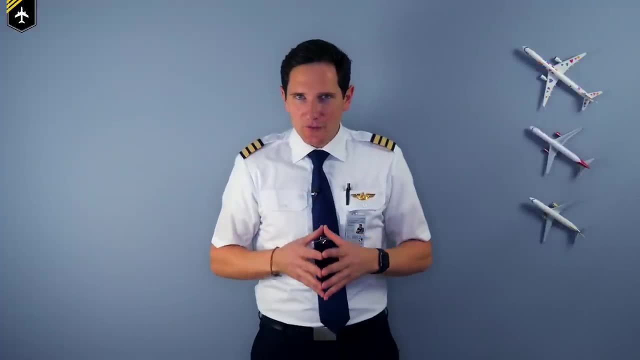 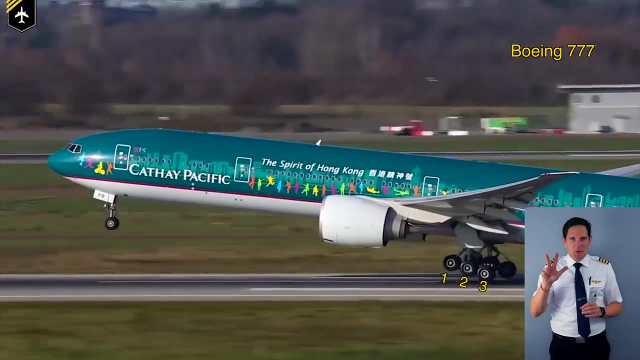 have a similar range and some airlines operate both aircraft, so how can you tell them apart? Now, one very easy way to identify them is by looking at the number of wheels and wheels, and remembering this simple quote: a Boeing 777 has a triple bogey. Take a look at the main gear. 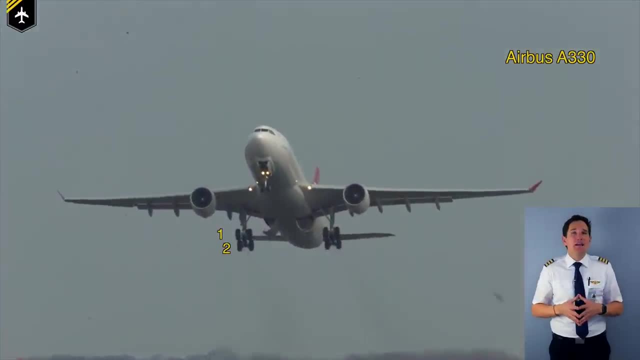 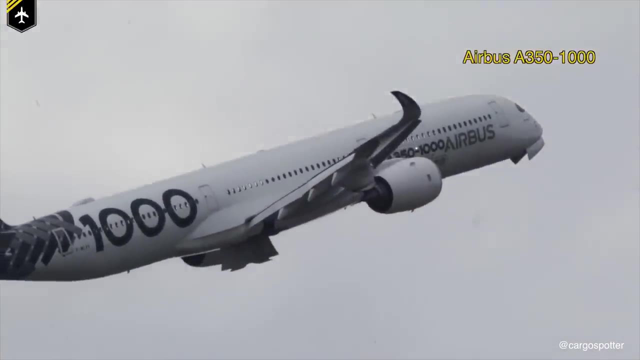 section of an Airbus A330, and you realize it only has a double bogey. However, don't get that mixed up with the more recent A350-1000, which also has a triple bogey. Now for this, you just have to. 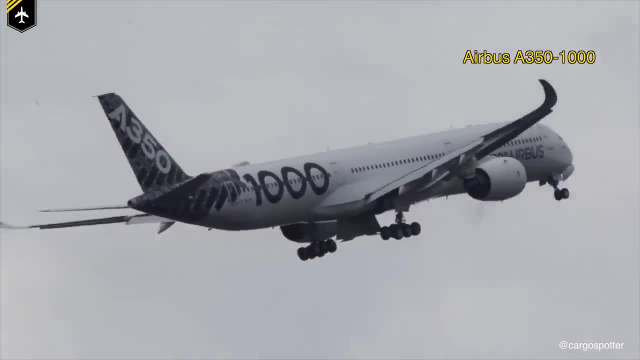 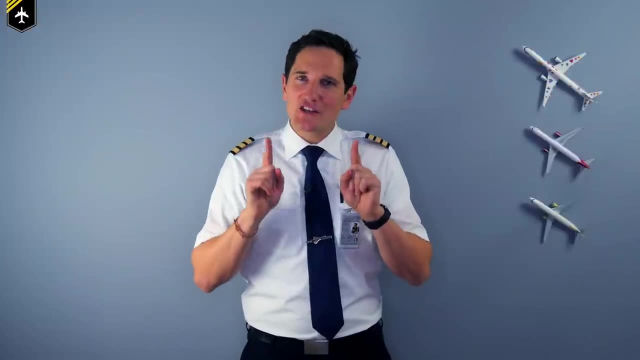 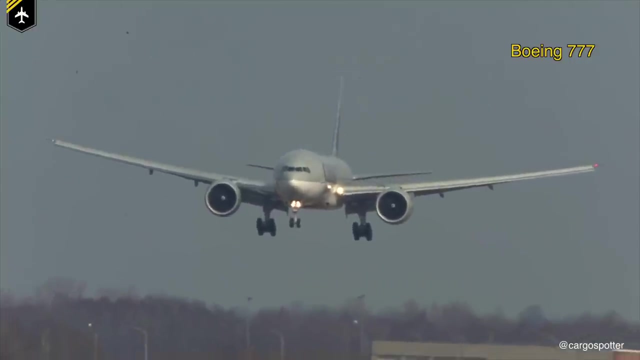 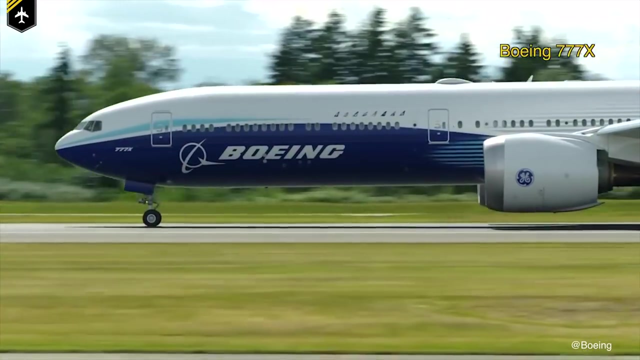 take a look at the wing tips to see those beautiful new Airbus A350 curved sharklets. Now, the one thing the 777 definitely doesn't lack, on the other hand, is engine size. These things are absolutely massive and with the new 777X soon to be released onto the market, they will take off. 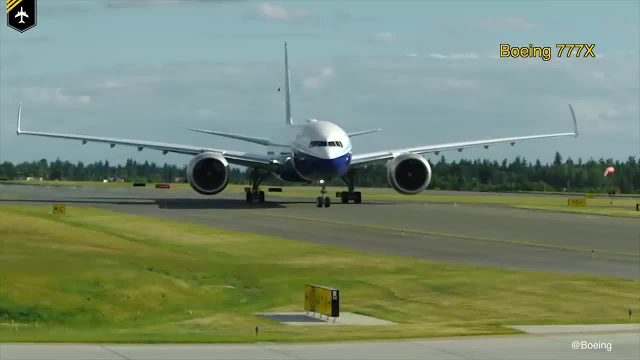 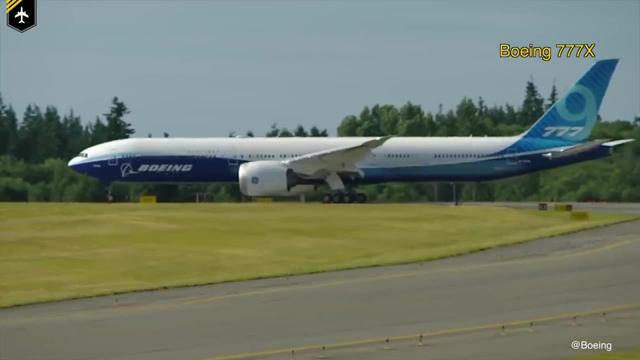 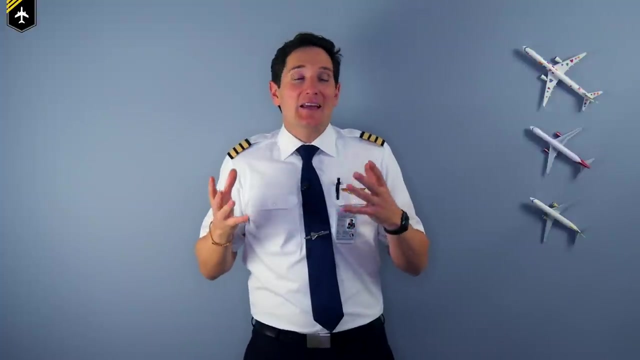 into the sky with the biggest and most powerful commercial engines ever produced in history. Now, to put this in perspective, the fuselage of a 737 can fit inside the engine of a 777X. Okay, on to the real big ones, or the heavies. So spotting the difference between a 747 and an Airbus. 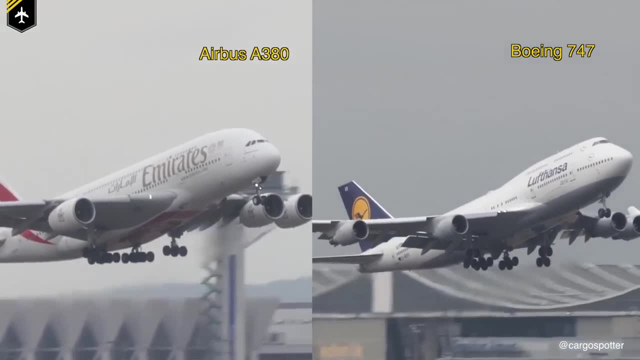 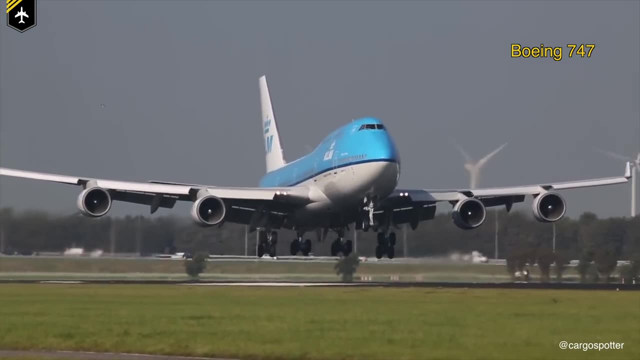 A380.. What could be easier? All you need to do here is to take a quick look and if it's big, beautiful, gorgeous and it looks very elegant, you'll have your answer straight away, because, of course, it can only be none other than the 747.. 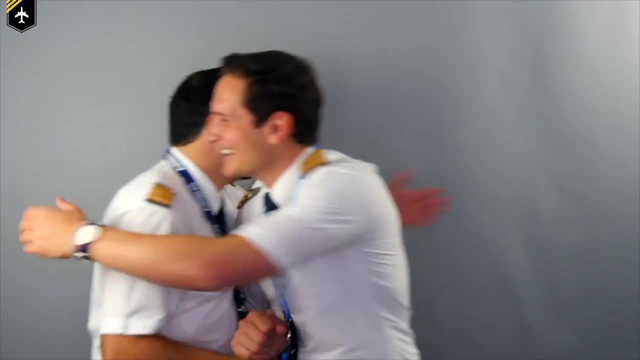 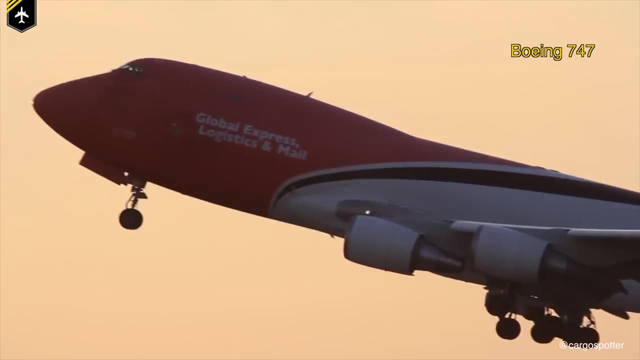 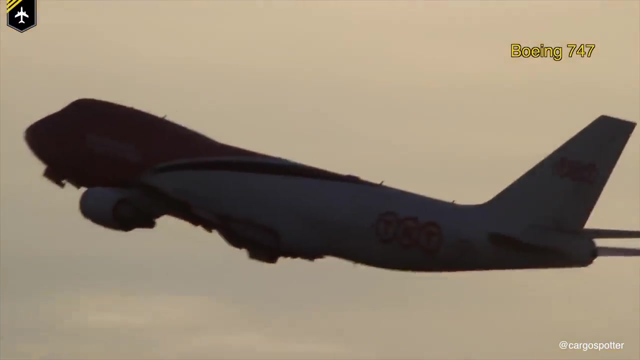 Pilot Alexander obviously disagrees with me. Jokes aside, although these are both four-engine aircraft, the easiest way to see the difference is taking a look at the upper deck. You'll see that all 747 models have the famous hump that makes up one-third of the aircraft. and compared to the Airbus A380, with its full-length upper deck. Also, if you want to spot the difference between a 747-400 and a 747-8, just check. the 400 has winglets and the dash 8 doesn't. Also, the dash 8 is a little bit longer. 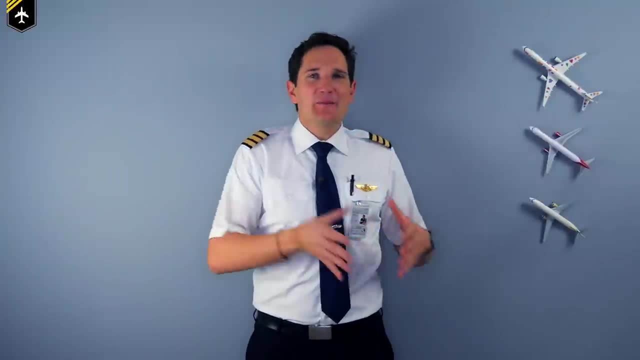 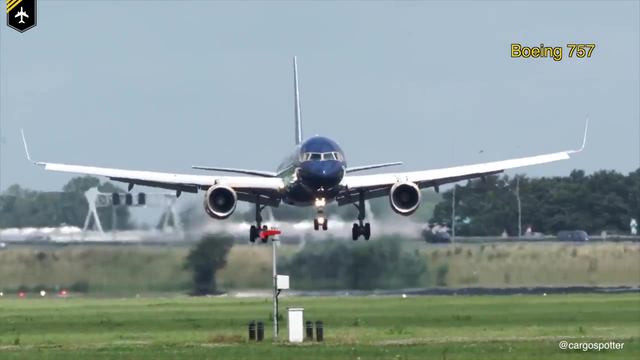 So we've talked about the little ones, we've talked about the large ones, but what about the ones in between? For example, the Boeing 757 is often referred as the flying pencil, and it isn't hard to get wrong. It's skinny, a single-arm fuselage and those strangely 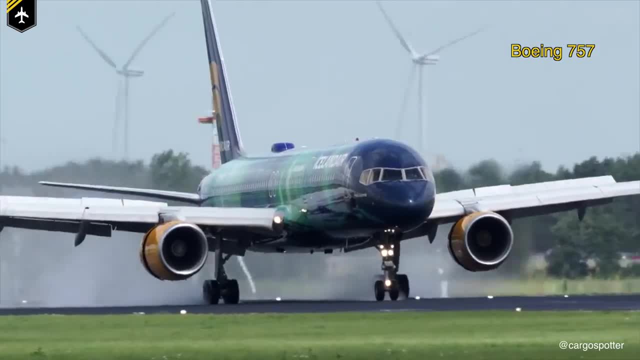 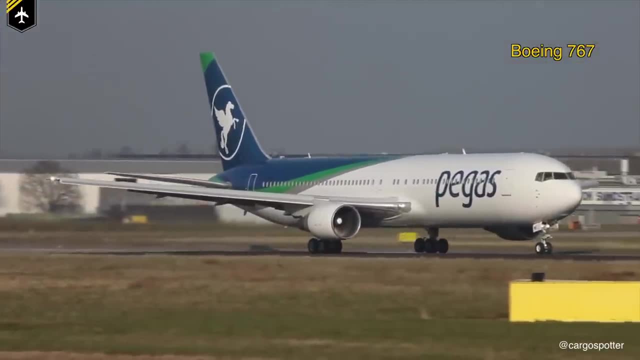 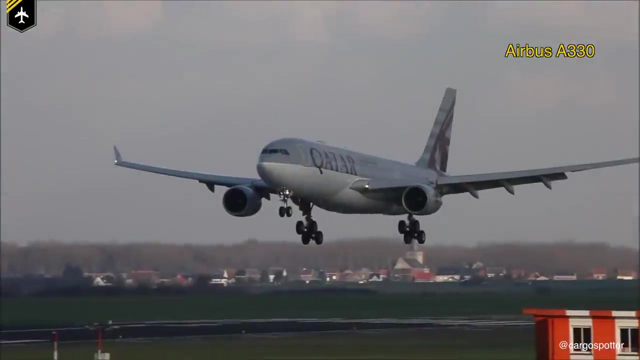 high landing gears gives it its famous name. But what about her sister, the 767?? The 767 is very often mixed up with the Airbus A330.. The simplest way to distinguish the two of them is by watching them both land. You'll notice that the landing gear of the Airbus A330 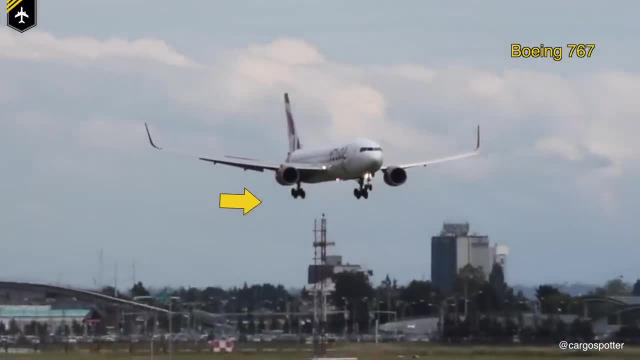 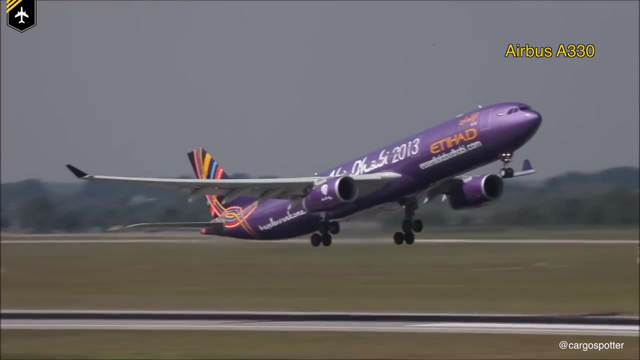 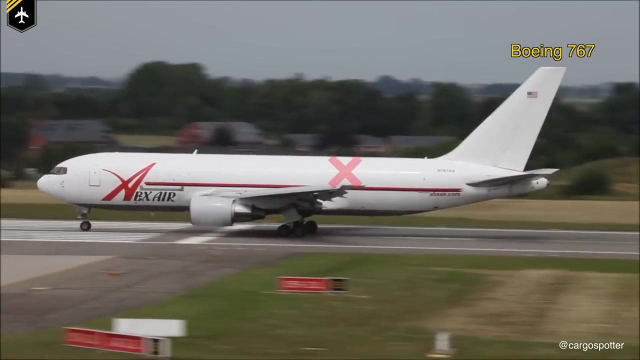 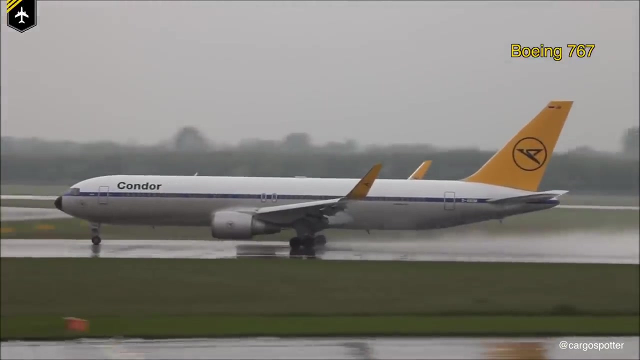 tilts backwards, with the Boeing 767 being one of the rare aircrafts to feature a forward-tilting landing gear. To add, the Airbus A330 has these small sharklets which come off the wing at a 45-degree angle, And the 767 often doesn't have any winglets, but if she does, they are humongous and are attached. 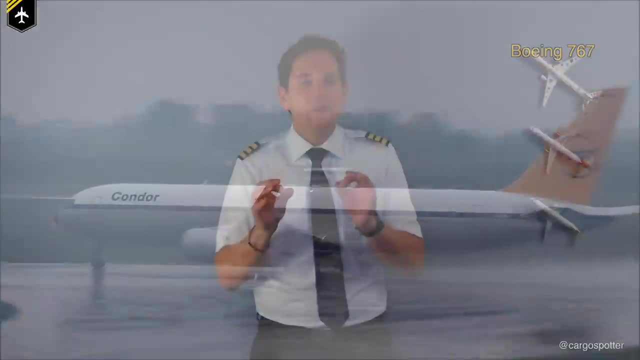 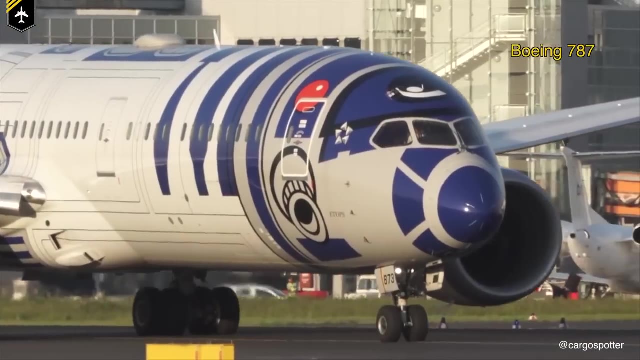 at a 90-degree angle to the wing. So keep your eyes out for that when you're boarding on your next trip. If you're struggling to see the difference between these brand new super efficient twin-engine long-haul jets like the Dreamliner and the Airbus A350,, there is help. 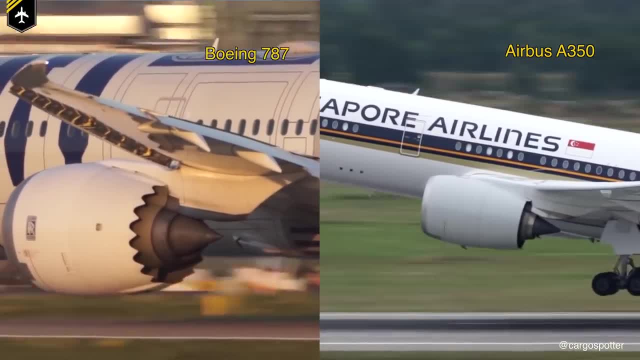 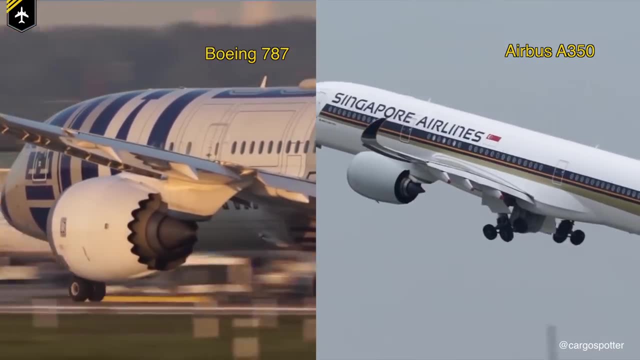 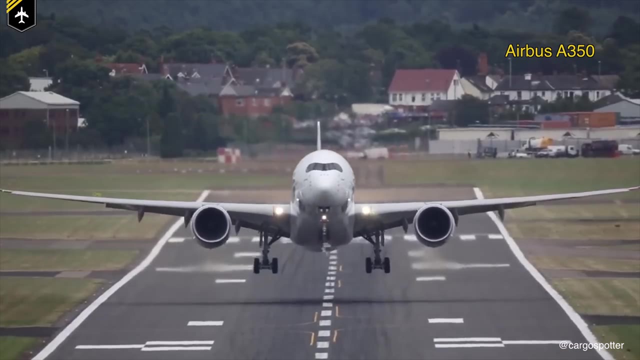 If you have a good side view on both of them, you will immediately see the Dreamliner's famous chevron nozzle at the rear of the engine cowling. Now, those curves are not just good for looks. this helps reducing the overall noise of the engine. The newer A350 doesn't feature this. 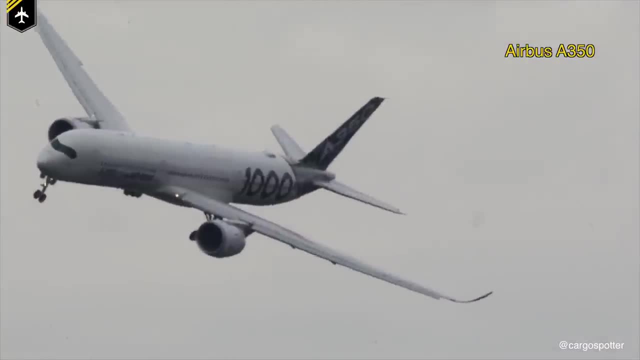 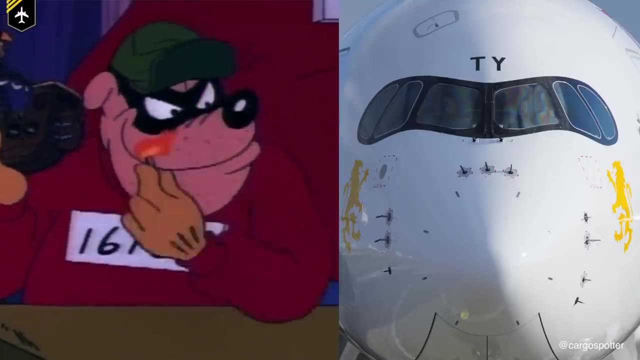 design and has managed to reduce its noise levels by other means. Also, doesn't the Airbus A350 from a front perspective remind you of the Beagle Boys from the DuckTales? You'll remember that the next time you see an Airbus A350 that I said that. 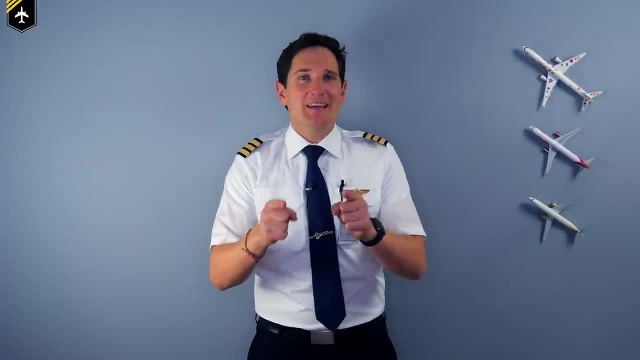 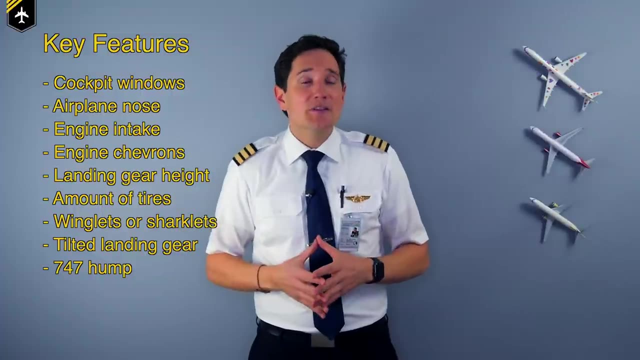 So some of the Airbus A350s that I've shown you in this video are the same as the Dreamliner. Now, these mentioned features will help you identify if you are either flying on an Airbus or a Boeing. Now, most of these features are either aerodynamical improvements over the years. 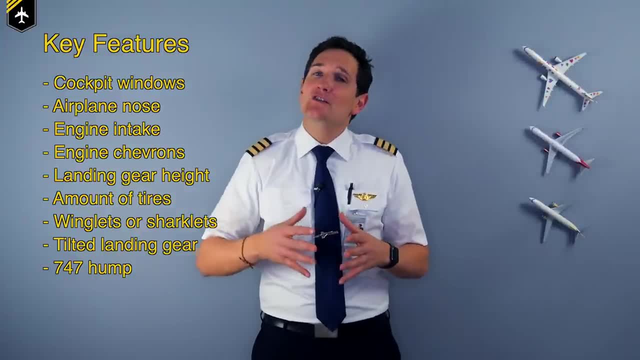 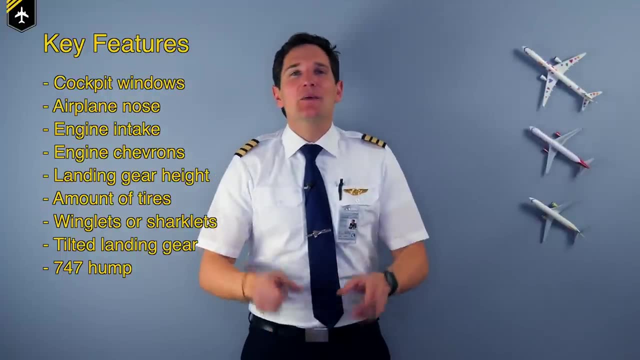 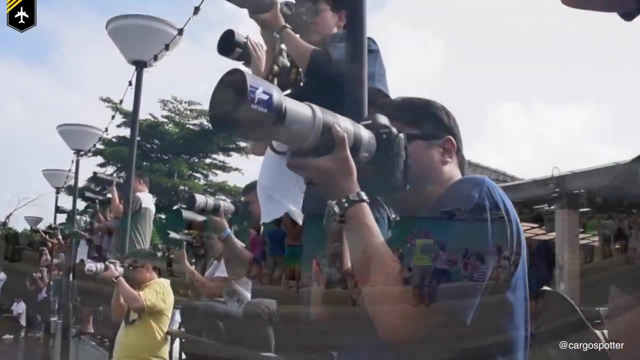 manufacturing quirks by the engineers, noise reduction, enhancements or just coincidences. So remember a couple of those little tips I've just given you and you'll be well on your way to compete with those super knowledgeable plane spotters. And maybe even the next time you're going on holiday you can impress your mates. 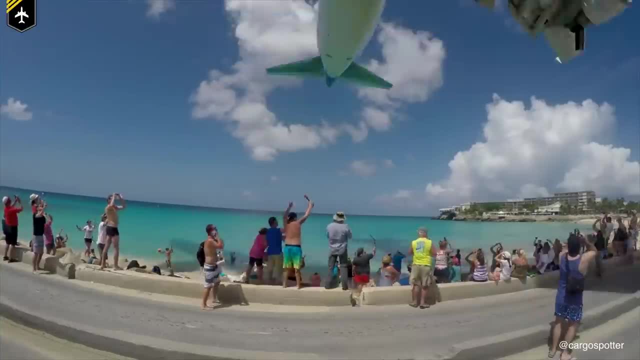 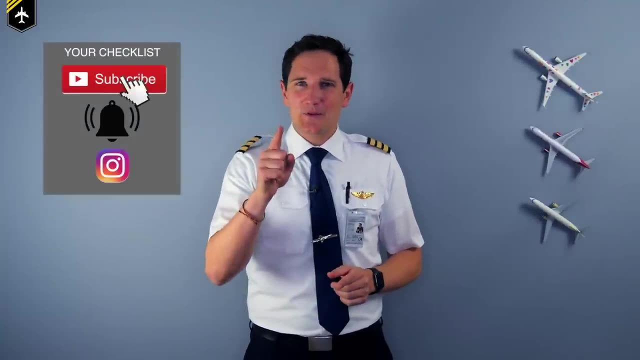 and family with this new found knowledge. Therefore, share this video with your friends and family. That's it for today. Thank you very much for your time. Here is your checklist. Subscribe to my channel. Check, Activate the notification bell. Check And follow my Instagram.